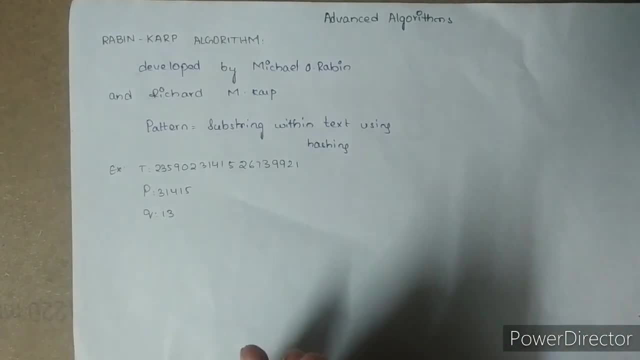 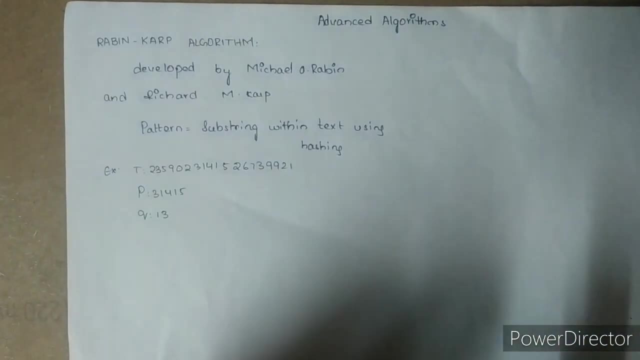 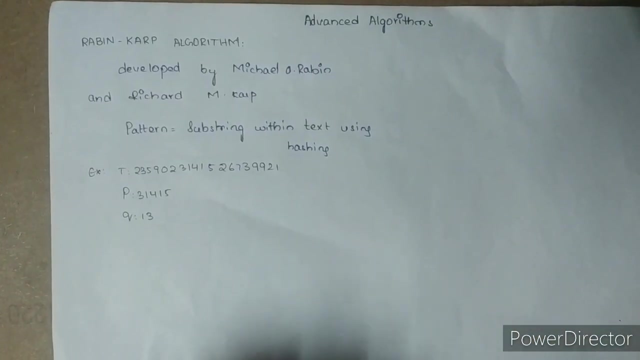 what is the main point here is we are using hashing. With hashing we are doing the whole problem. So what? the same process, the same process was same, And in this what we will do is only hashing will be different. And by what? hashing is nothing but doing making the longest. 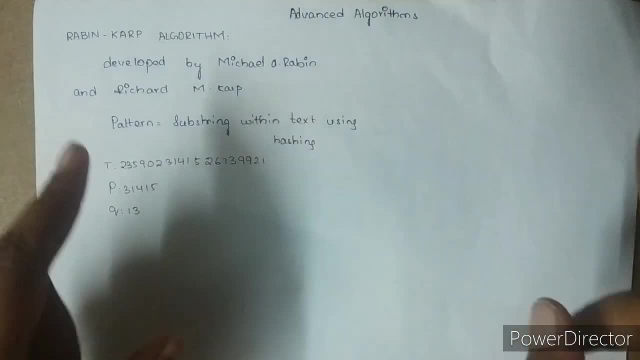 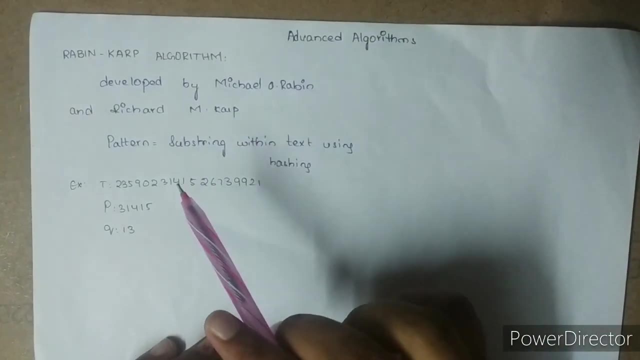 means longest string into short string. Yeah, this Rabin-Karp method was developed by Michael O Rabin and Richard M Karp. These two were developed. this one, So this algorithm got Rabin-Karp. So this algorithm got Rabin-Karp. So this algorithm got Rabin-Karp. So this: 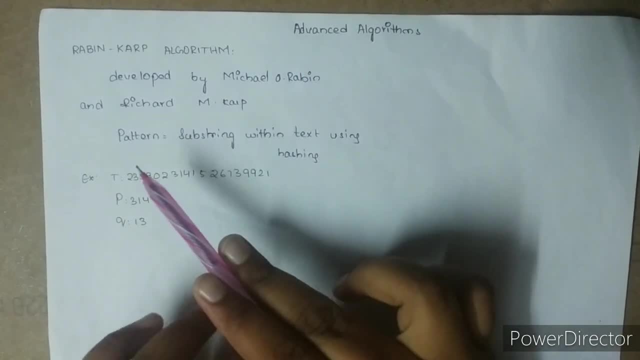 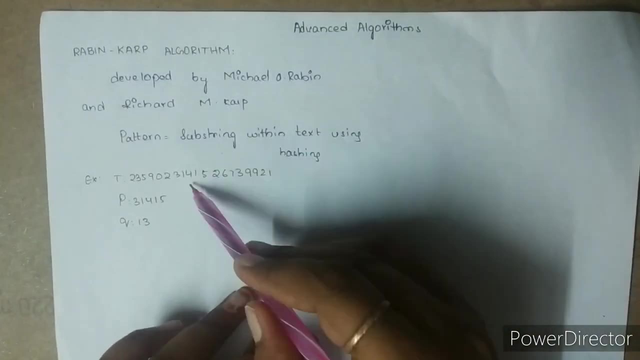 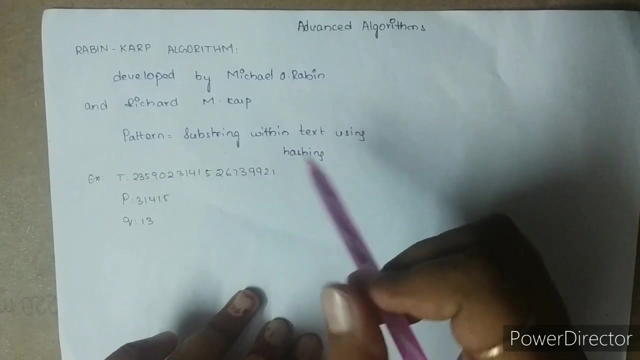 Rabin-Karp algorithm In this pattern is equal to substring within text using hashing. The substring pattern is a substring. If you have these old string in that the only point, this one is a substring and this is got by using hashing. So let me explain this with. 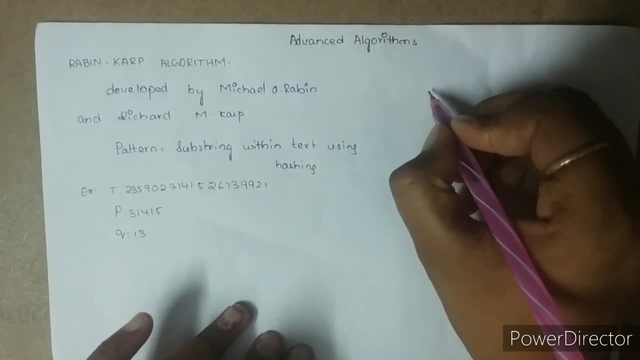 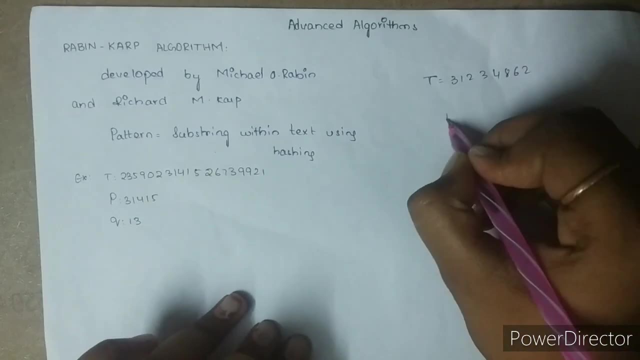 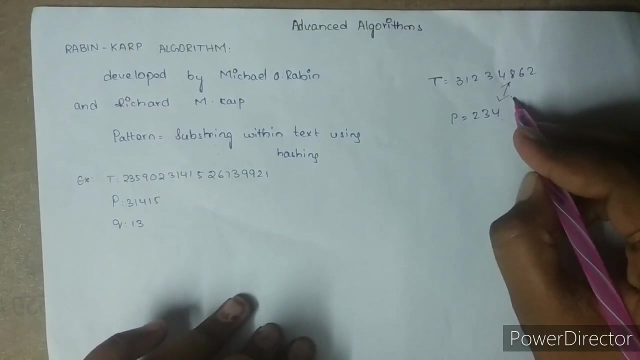 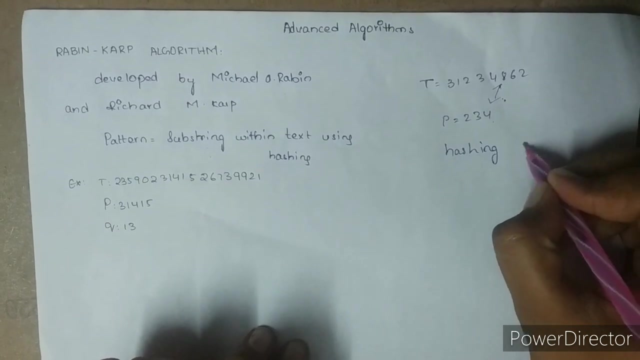 an example here. The example is- let me take an example: t is equal to 31234862.. And the pattern will be 234.. Here to check whether these two are getting matched. what we are doing is hashing right Hashing. Hashing is taken by Q And this Q value what we are. 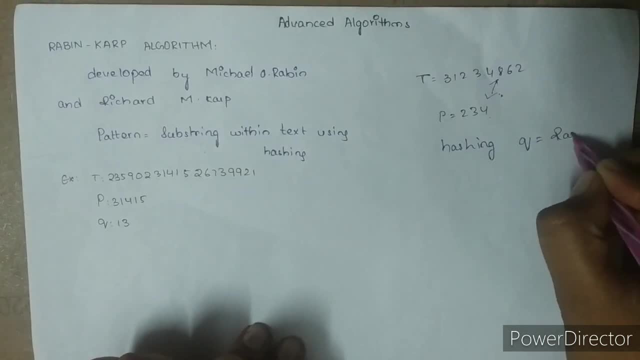 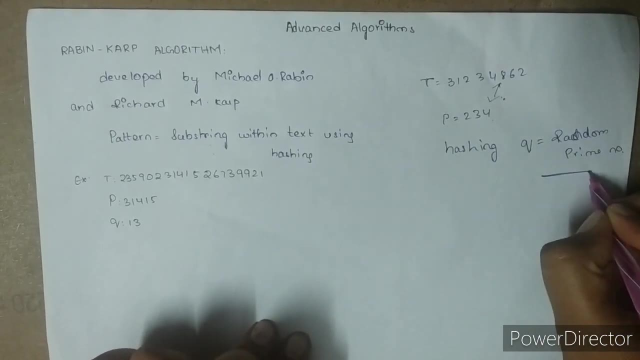 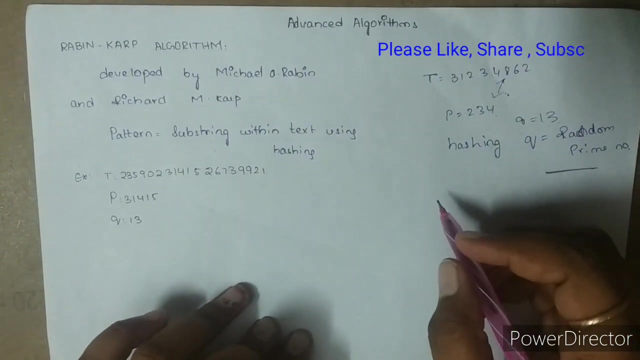 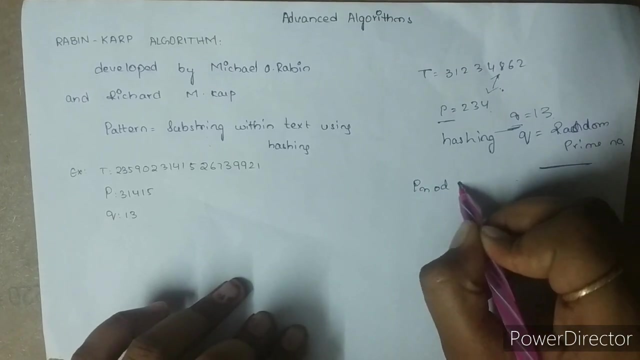 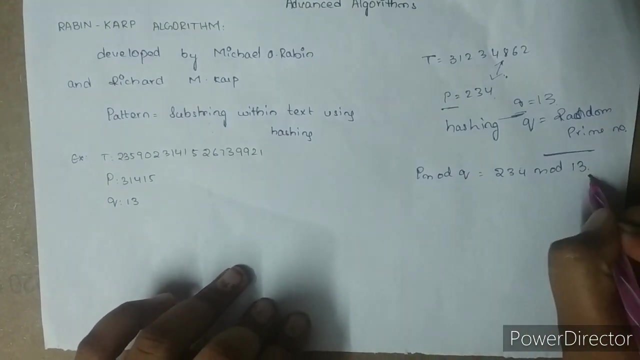 taking the Q value is the random prime number. We can take any random prime number. Here. I am taking Q is equal to 13,. right, Let us start hashing here. First we should check P and Q hashing. So P mod Q, What P mod Q is 234 mod 13.. The value of 234 mod 13 is 0.. This was calculated. 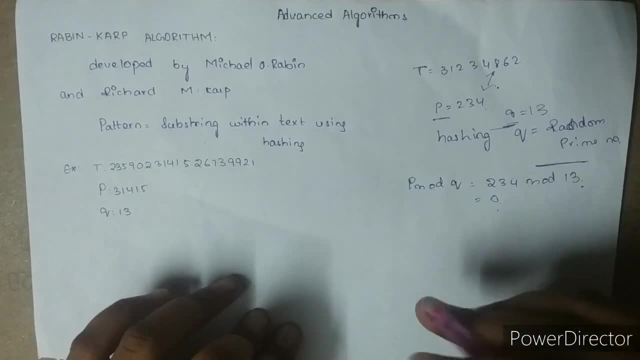 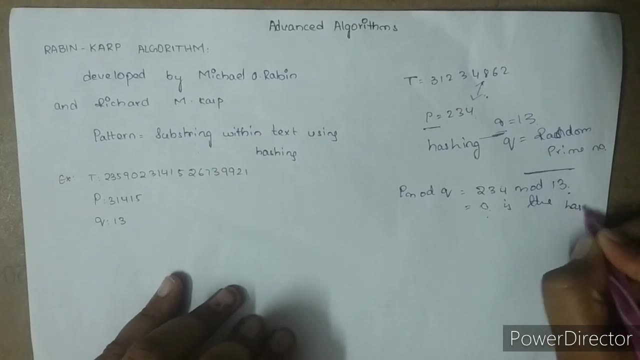 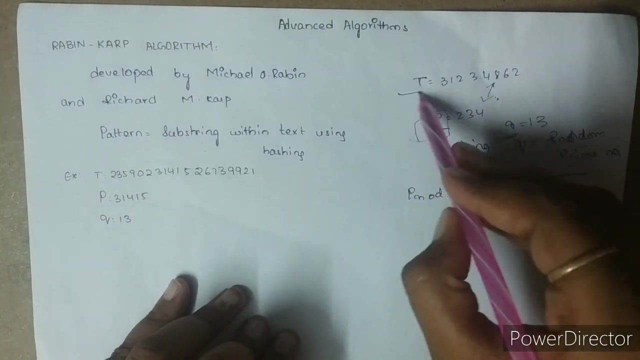 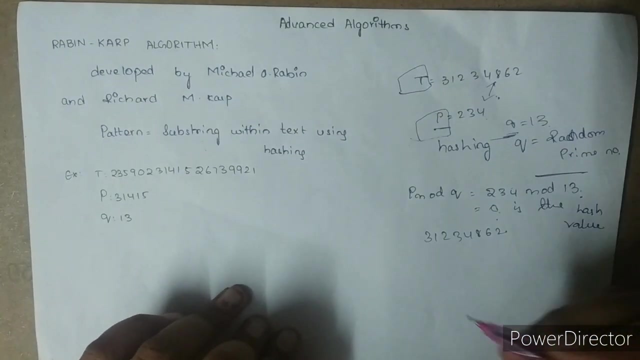 from scientific calculator. If you have scientific calculators you can calculate in there. And here 0 is there. This is the hash value. So first I have calculated hash value for P and now I am calculating hash value for T. So let me take the values here. First we should check how we are doing. 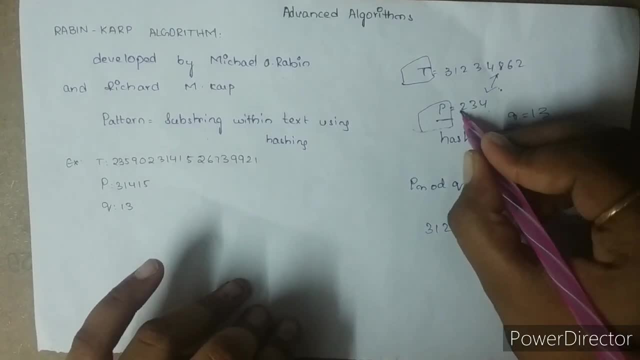 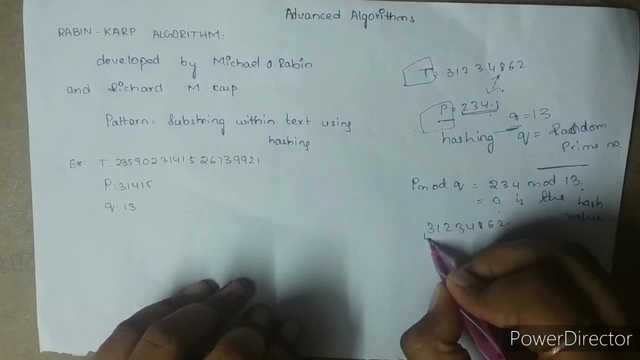 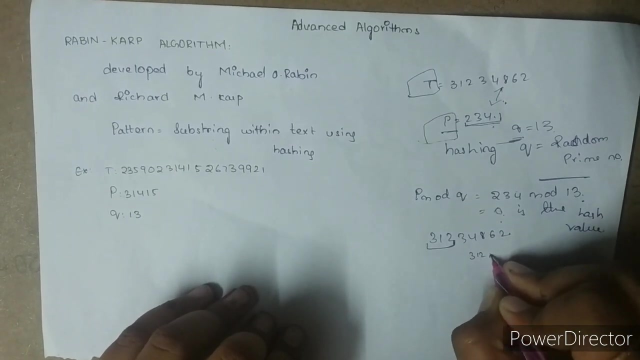 hashing here. Let us see first how many values are there in pattern And then check the text value. Same number of values: we should take here 312.. These are three values and we should take here also three values. So 312 mod again. 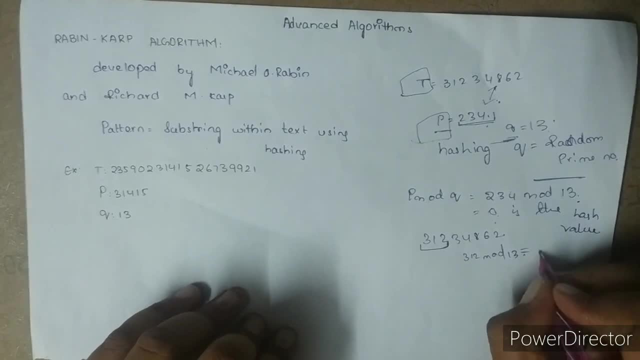 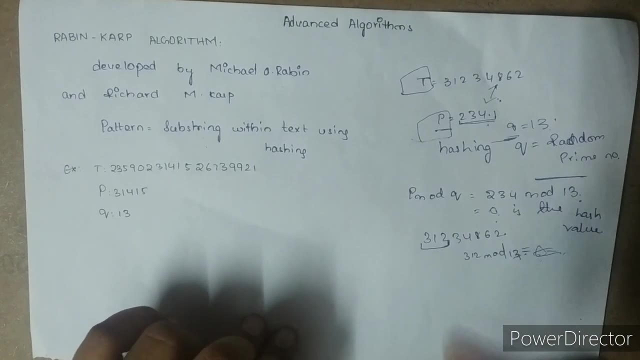 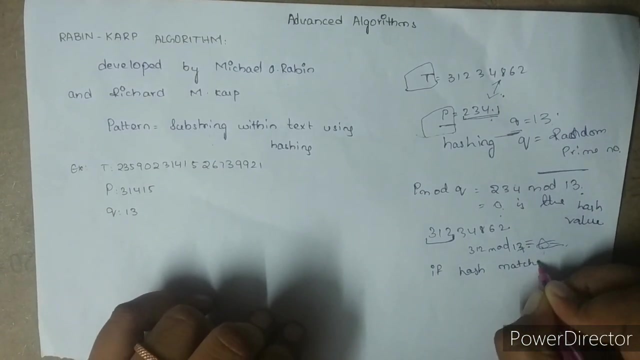 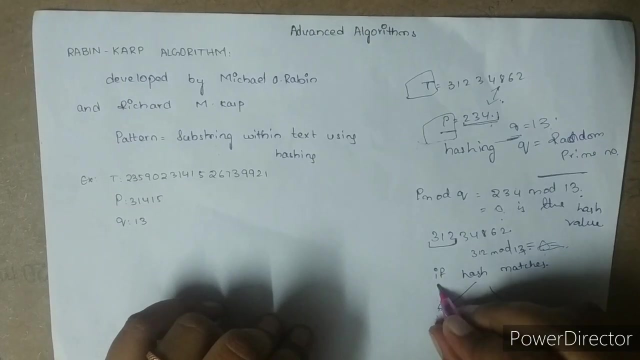 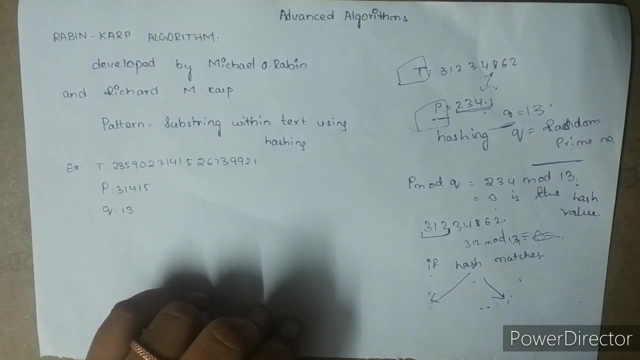 13. 13.. The value will be what we calculate here And here. what I want to say is here we have two points. If hash matches- Yes. if hash matches First step, two problems will get Yes. if hash matches two answers, we will get Matching right. let me explain. 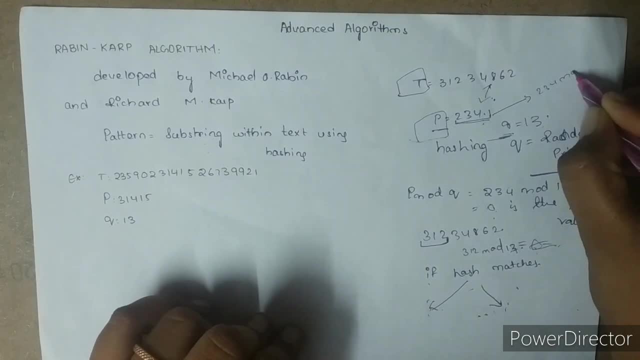 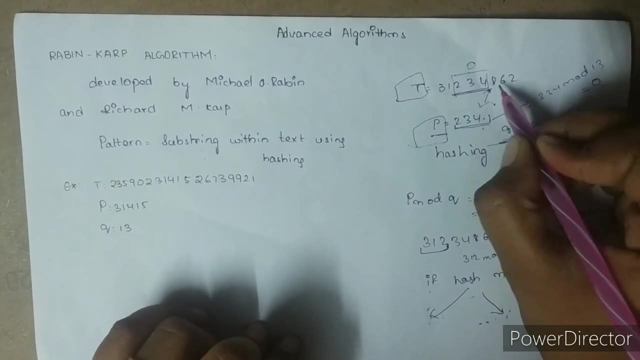 in this only, We have got 234 mod 13,. right, This value is 0.. And here is the value 234.. This value will be 0.. If the 0 value again comes with this value also, then what is the? 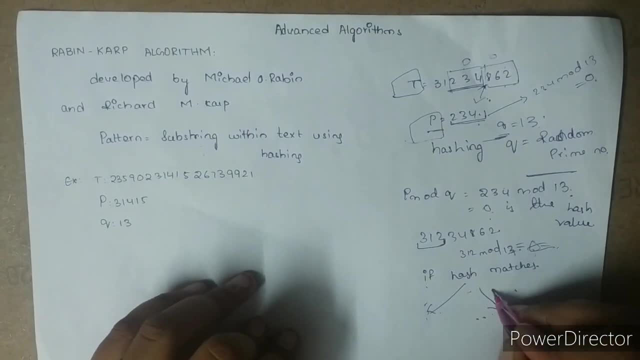 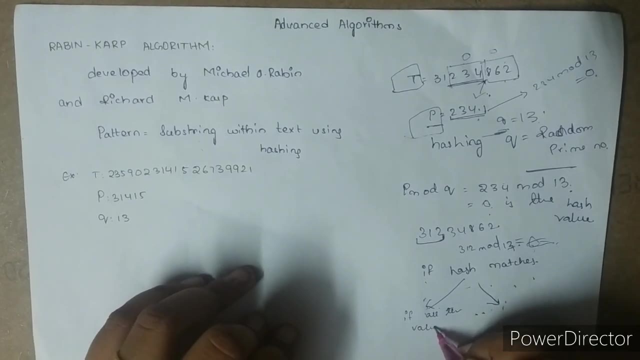 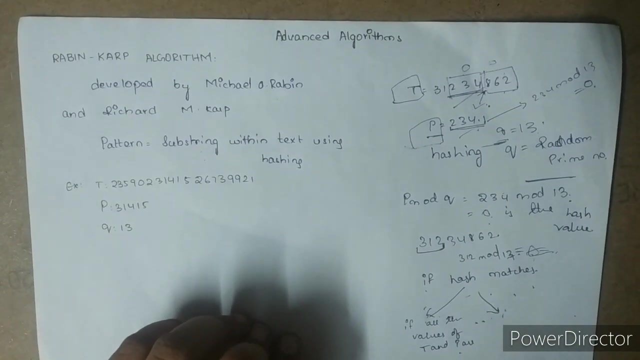 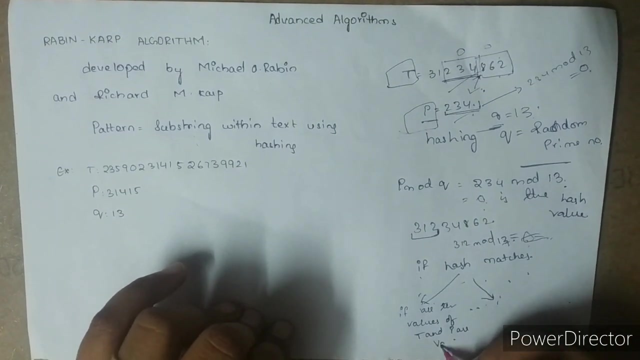 solution. Let us see here: If hash matches, So if all the values are matched, Values of T and P are matched. So like this, This 234 and this 234.. If two values are matched, then what is called as valid hit If these two? 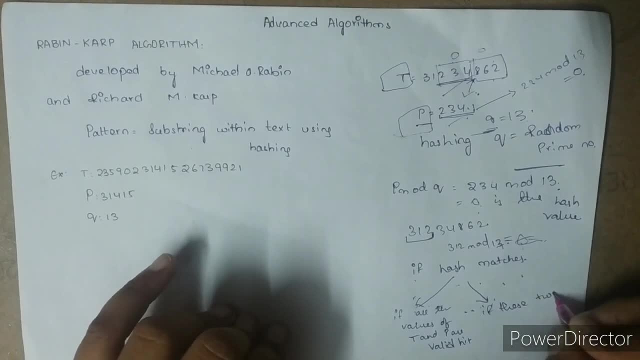 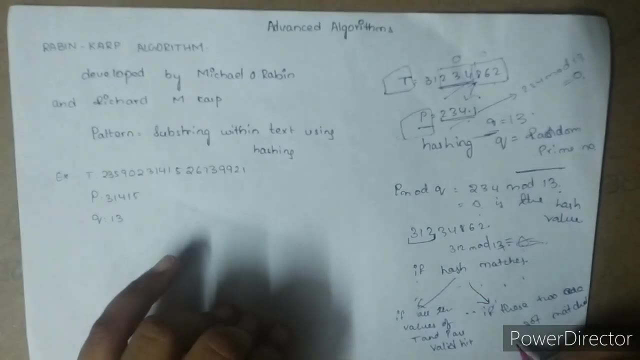 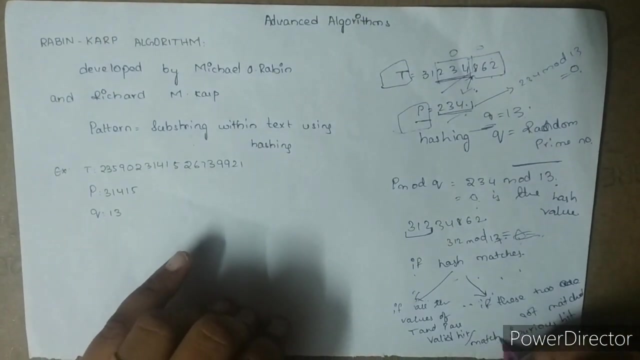 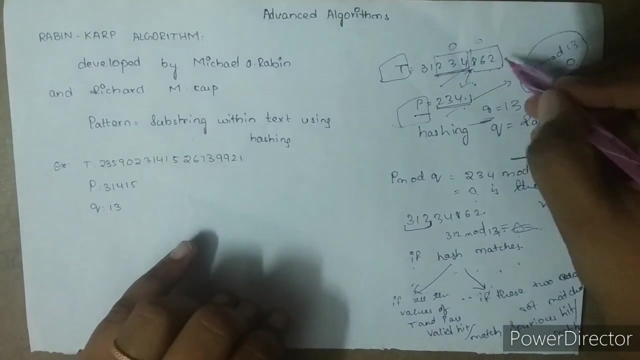 are not matched- These two are not matched- Then this is called as spurious hit. So this can be also called as match. Yes, valid match and spurious match. So here this is called valid match and this will be spurious. 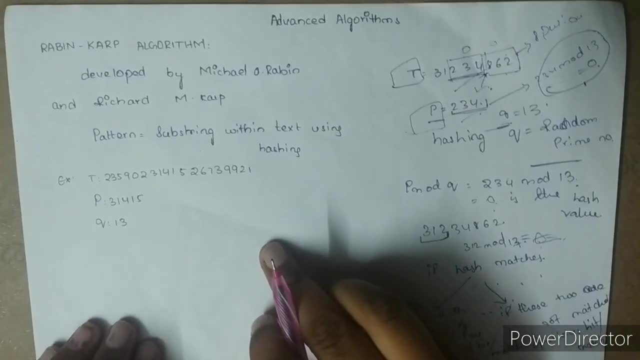 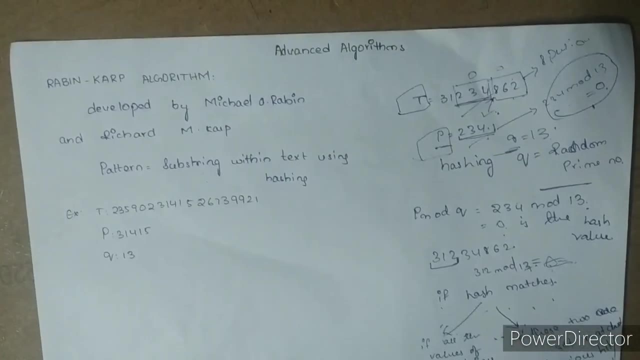 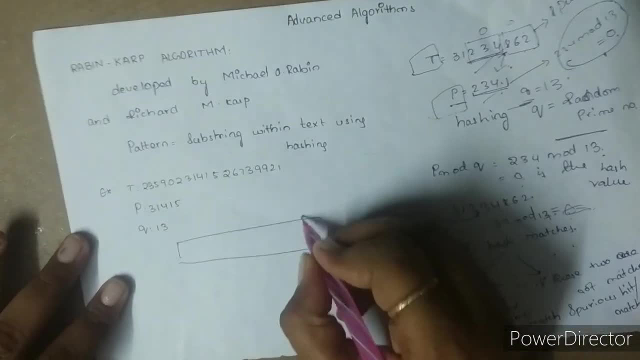 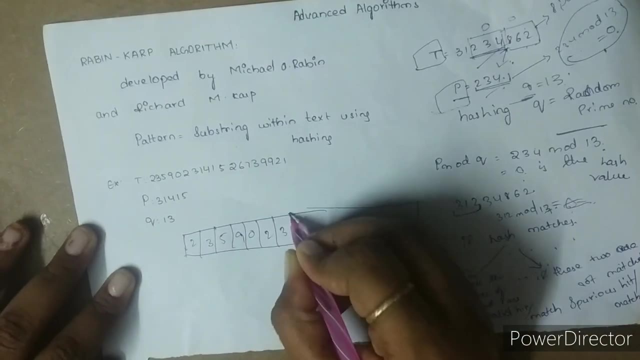 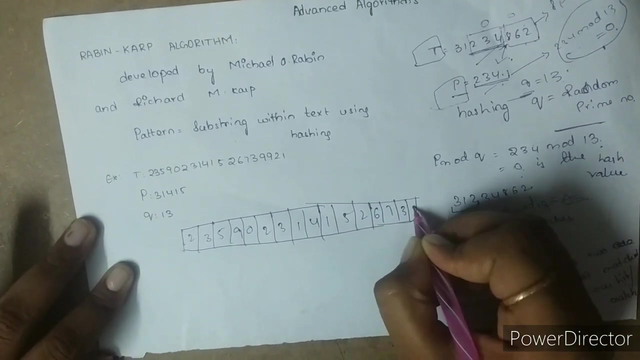 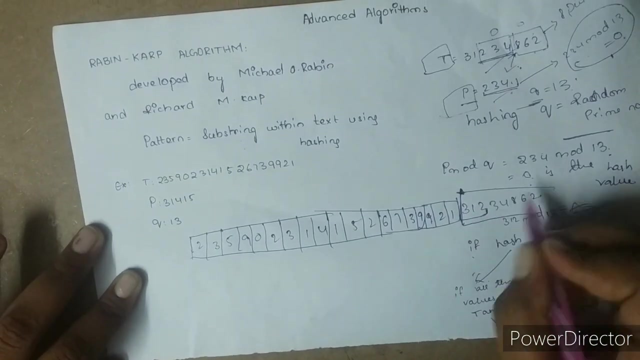 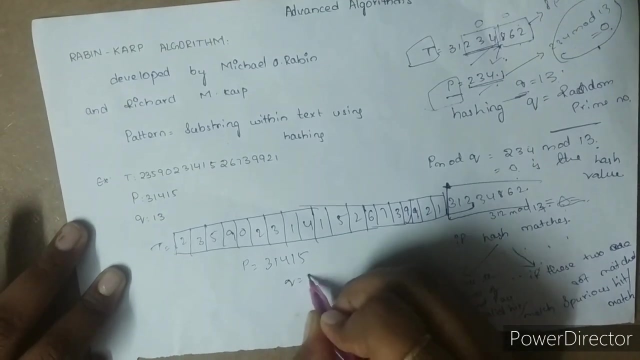 the block. the block will be like this: yeah, this is the value. so here, t is equal to this and p is equal to 3, 1, 4, 1, 5 and q is equal to 13,. right, p mod q. what we'll do is p mod q. 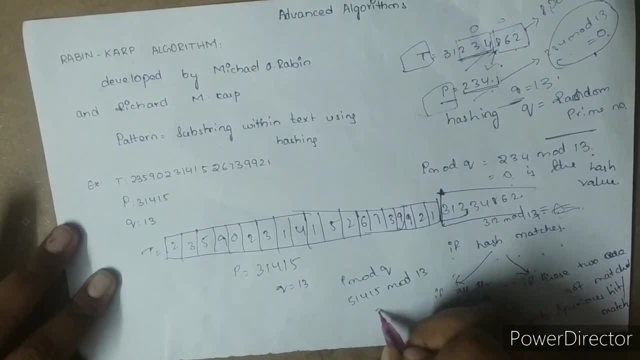 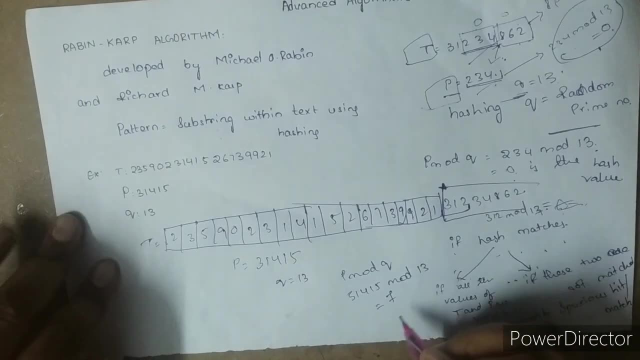 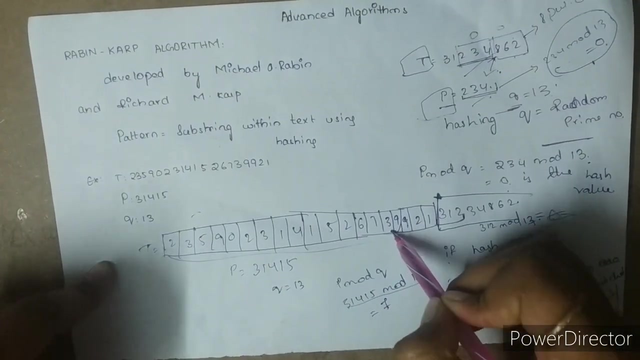 3, 1, 4, 1, 5 mod 13,. the value will be 7,. okay, the value will be 7 here. so here we should match this in this text. okay, pattern should come in this text. so first, how many values are there? 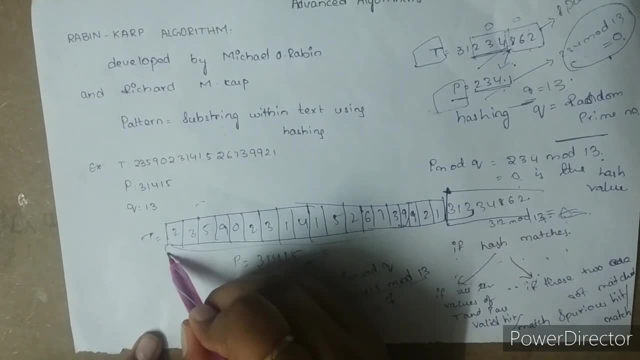 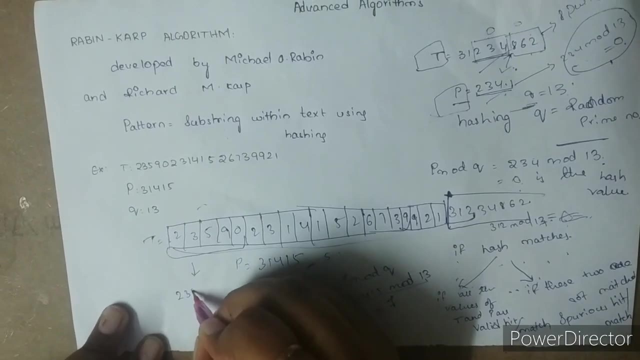 in pattern. let's check this. 5 values are there, so first 5, we should check first 5 values. what is the first value? 5 values match will be 2,, 3,, 5,, 9,, 0,, mod 13,. right, this value will be. 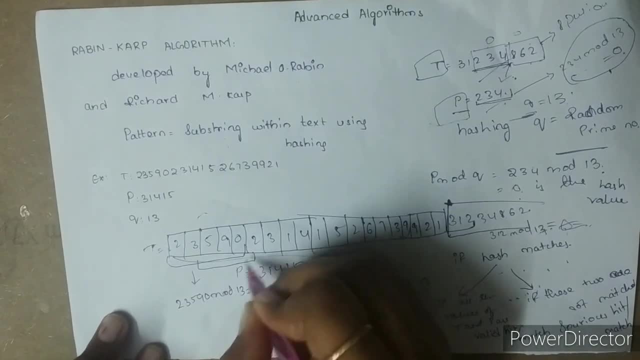 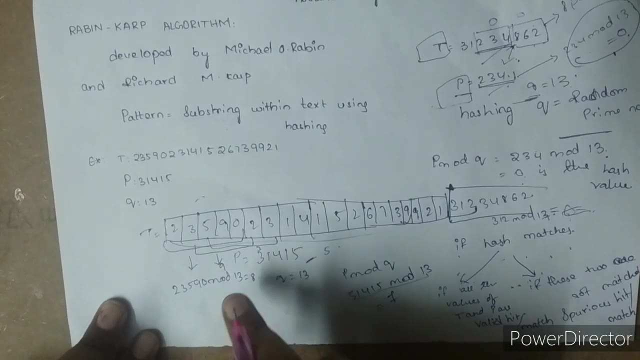 8 and the next 3,, next 5, next 5 values will be 9 and next 5 values will be 3, actually, before this video, I have calculated these values, so I'm writing it if you have any doubt. 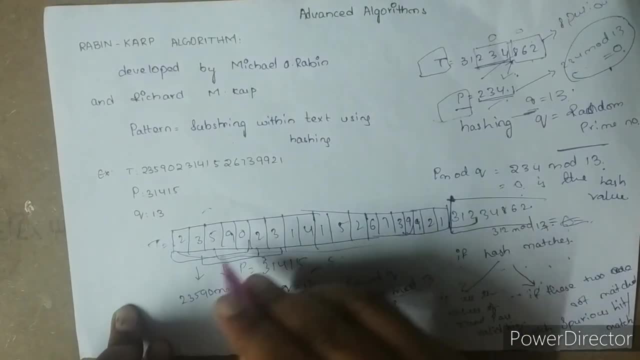 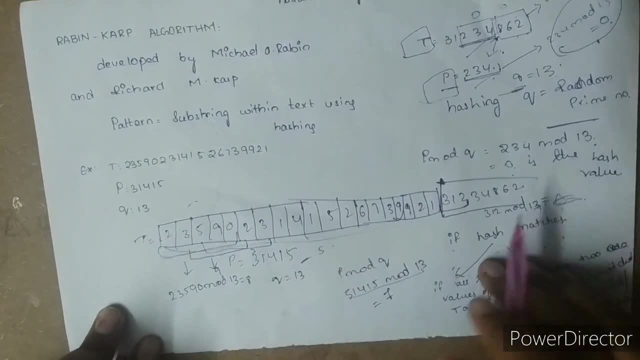 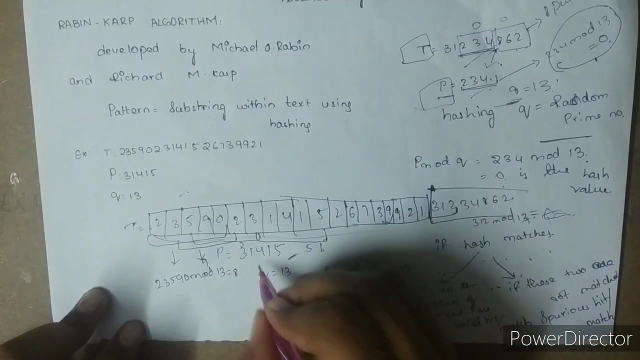 you can check there and while coming to this, we should check every one, every single block, we should check every single one, and then we take, we should take the values. so now I'm checking this: 3, 1, 4, 1, 5, what is this? 3, 1, 4, 1, 5, this is matched with this pattern and this value. 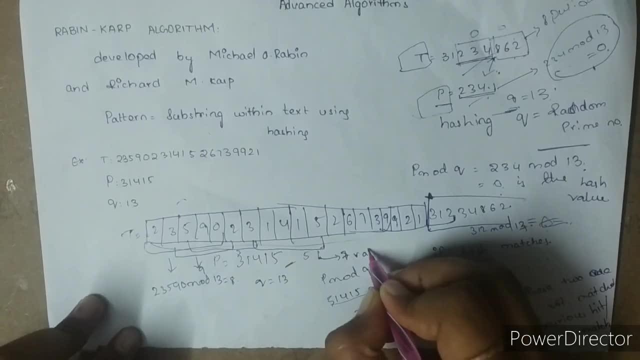 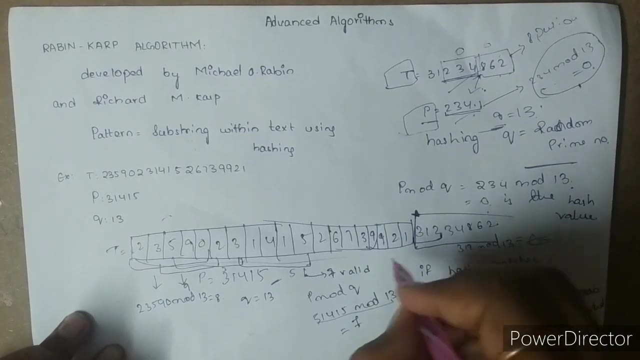 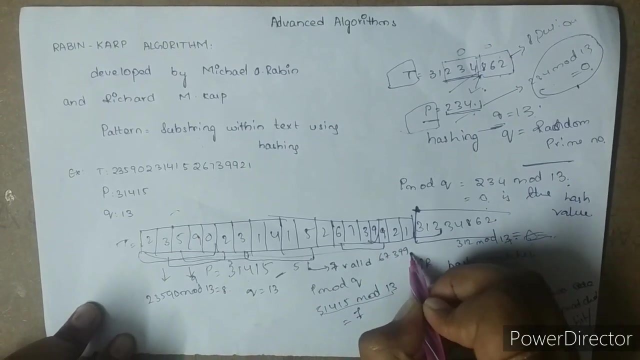 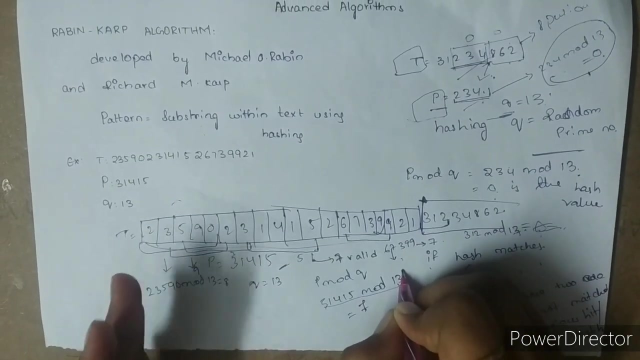 will be 7,. right, we have got valid hit and every some we have spurious hit also. so we have in this spurious hit. so here is the spurious hit: six, seven, three, double nine will also get the value seven. so this is the spurious value. so, um, we should check every single block, every single. 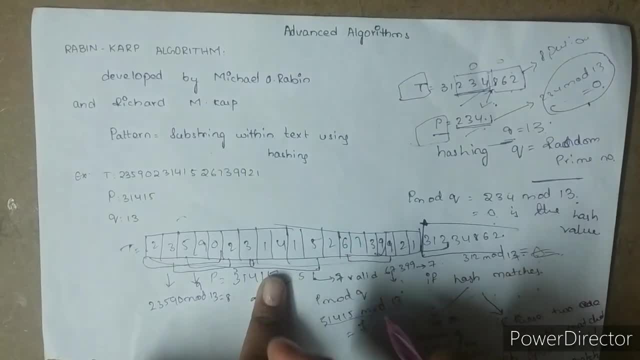 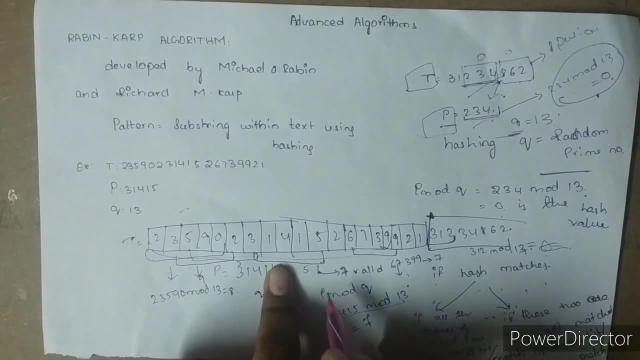 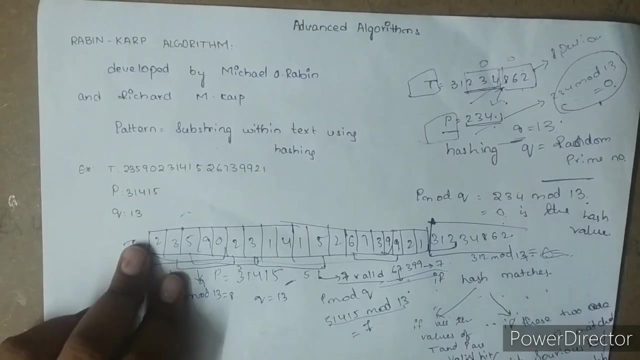 key right, every single key, and we should write a: uh, write as case one, case two, case three. we should do solve that problem. here we have got valid hit and also valid uh, spurious hit, so uh. this is the example, and now i'm going to explain you the algorithm of this problem. here is the algorithm. 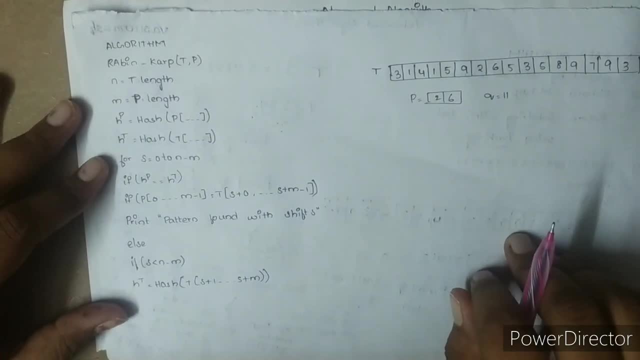 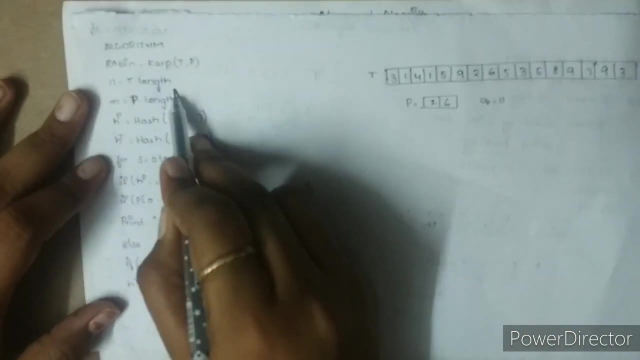 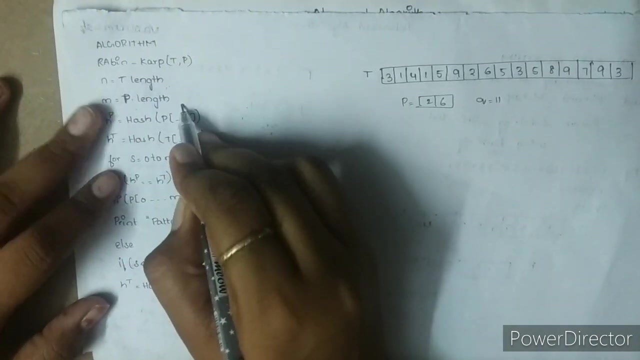 here is the algorithm. and in this algorithm, uh, let's check n, t length. n is equal to t length and m is equal to t length, p length, that is length of text and length of pattern, and what we are taking here is h per p equal to hash. 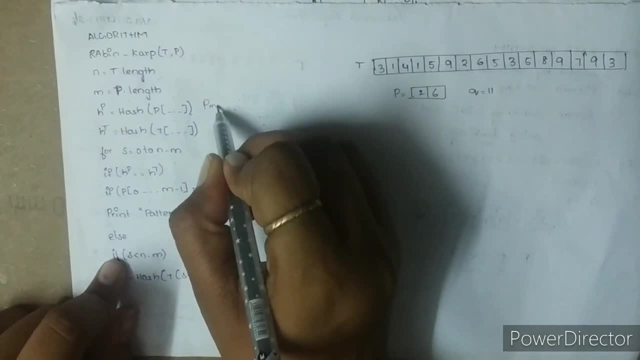 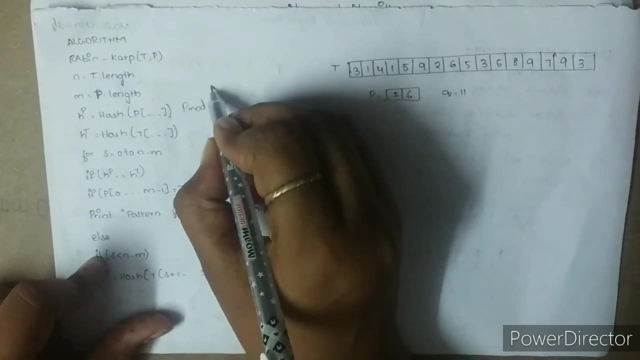 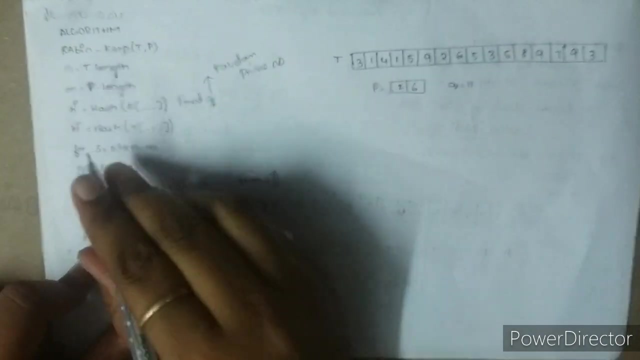 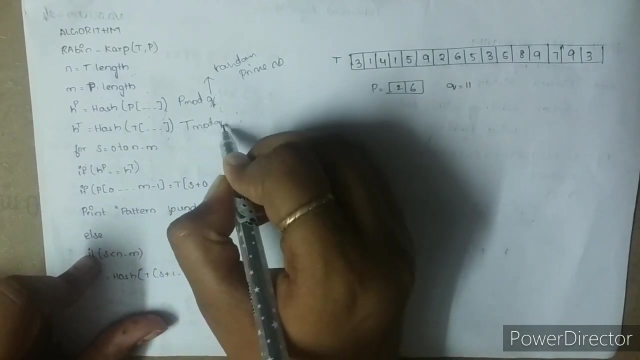 p value here this is called as p mod q. right, we are doing hashing for pattern, right here? p mod q and what is the q value? is random prime number, right, random prime number. and next one, h per t is equal to hash of t text, so this is called as t mod q and this is also called as random prime number. and to check whether 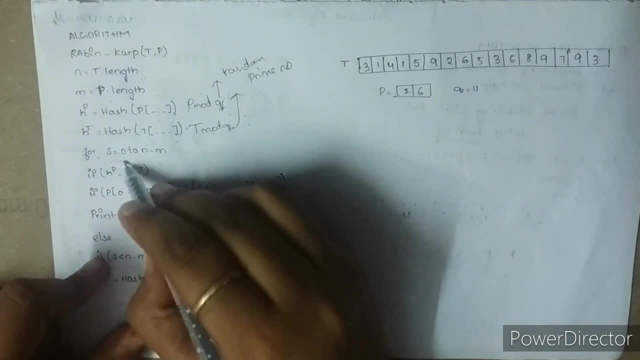 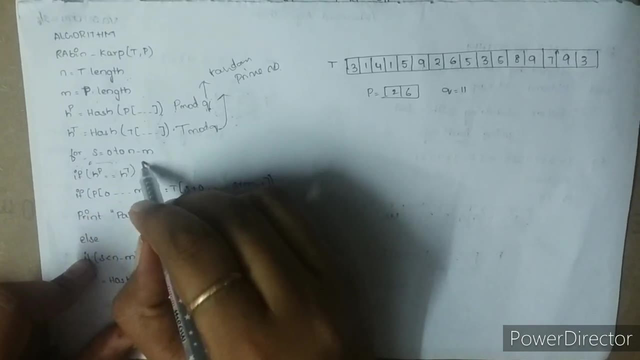 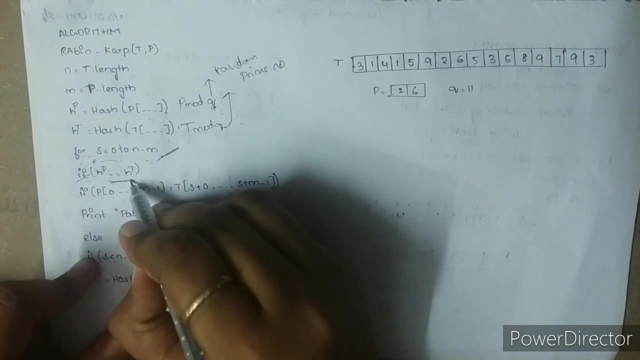 these are matching. we are using for loop to do shifts- right in the last video, have? we have seen this in the last problem also, if s is equal to 0 to n minus 1, and here is the another one. uh, if, if loop, this is to check whether these two are equal or not. pattern is equal to text or not, like. 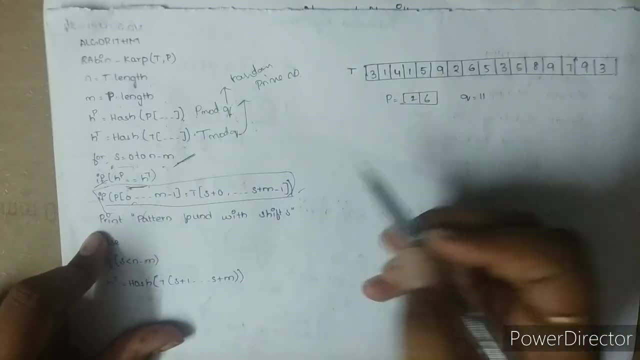 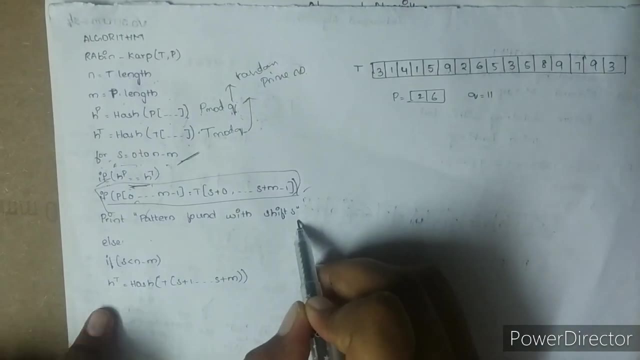 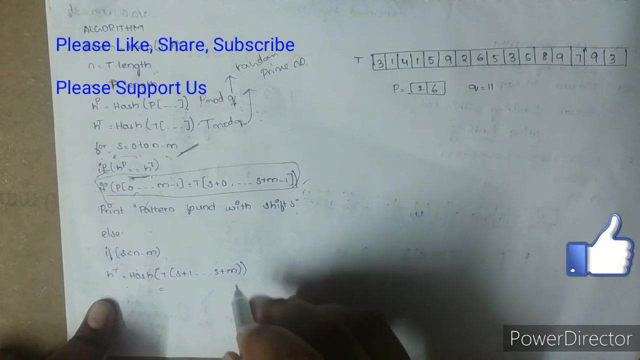 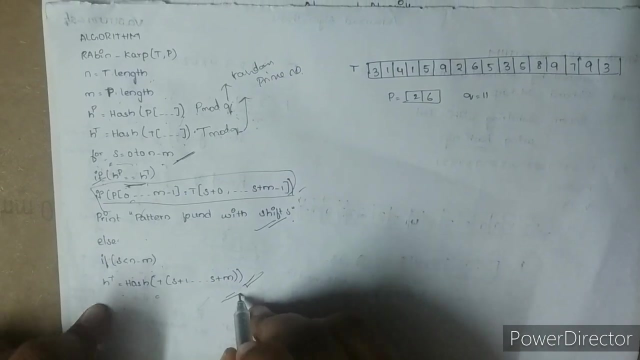 like this. we are going to check here and next. if we have matcher with the text, then what we'll write is: print is equal to pattern found with shift. if not, what we'll do? if s less than or less than n minus 1, then hash is equal to this. so if matches, we can write this. if not, it is not matched and 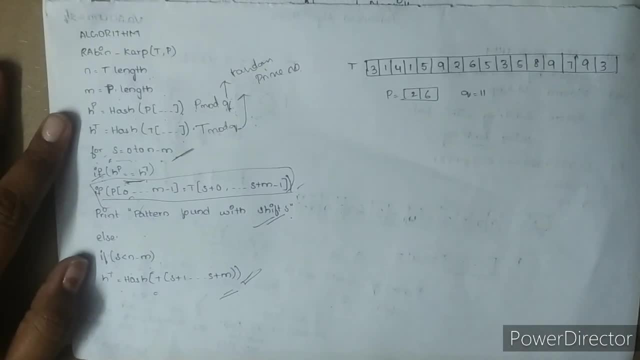 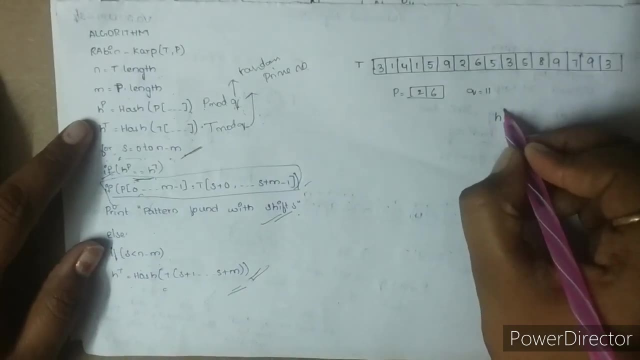 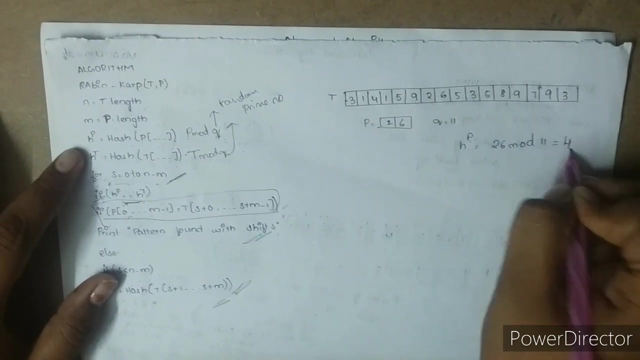 here is the another example for this problem and this example will be: uh, here is the example and here what i am doing is first what we do: hashing, hashing for pattern. so 26 mod 11 is equal to 4.. the hashing value of 26 mod 11 is 4, and 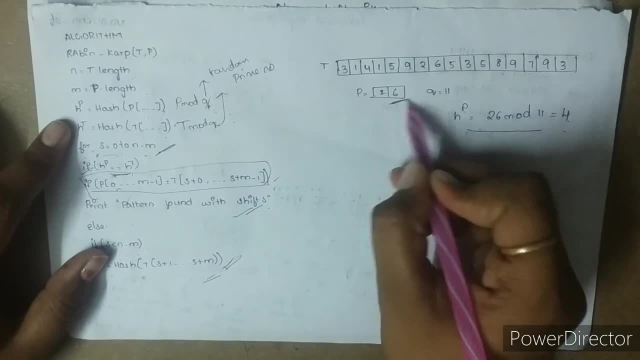 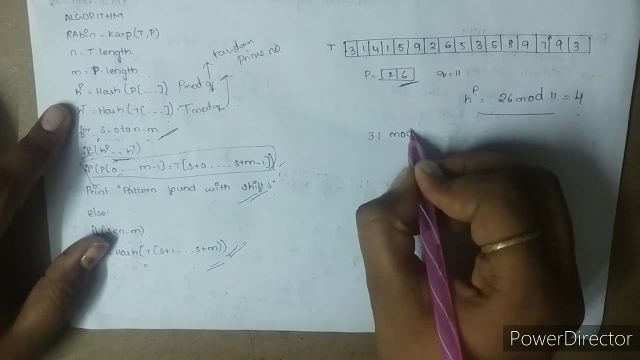 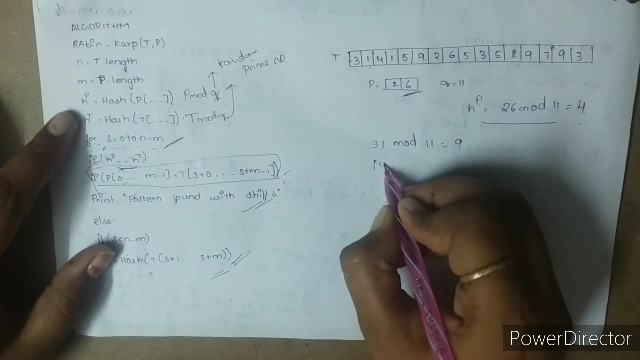 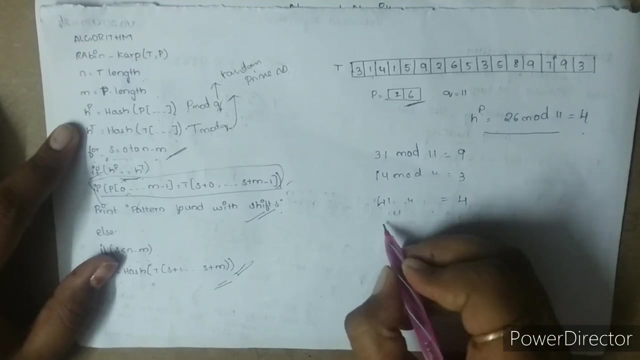 let me check for every single value in this. we have two values, so let first let's check 31, right, 31 mod 11.. this value will be 9 and next 14, 14 mod 11. this value will be 3 and 41- 41 value will be 4. sorry, 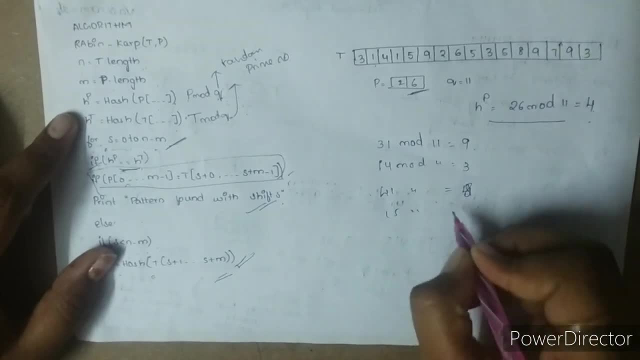 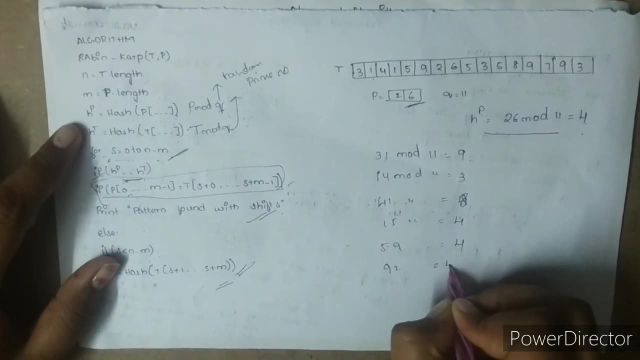 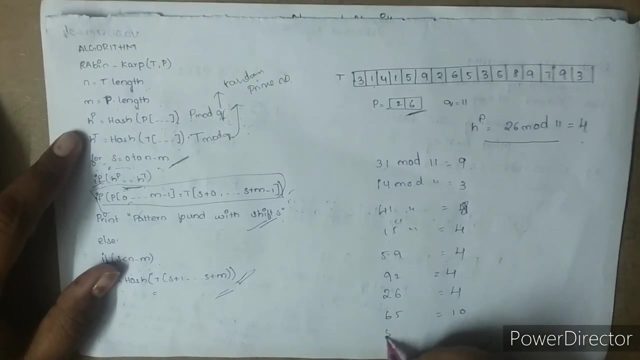 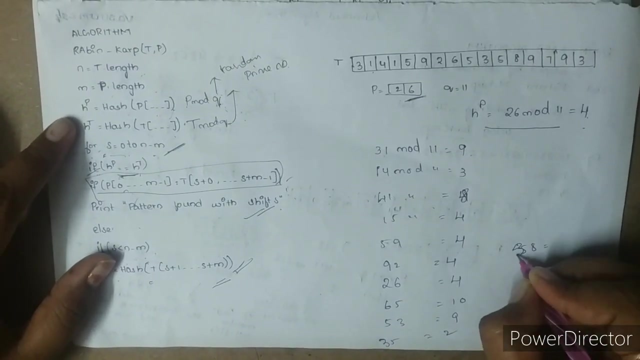 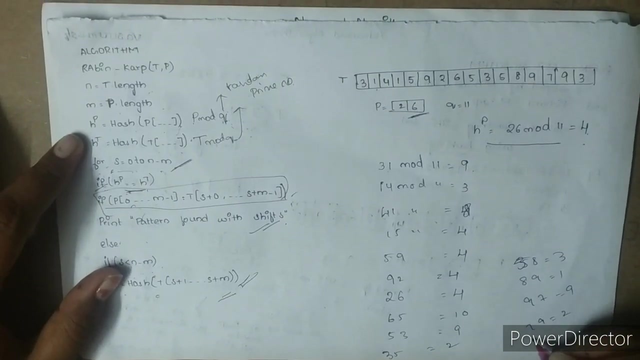 8 and uh 15. 15's value will be 4, 59, 59 value will be 4 and 92. 92's value will be 4, 26 value will be 4 and 65 is equal to 10.. 53 equal to 9, 35 equal to 2 and more. 58 is equal to 3, 89 equal to 197, equal to 9, 79 equal to 2 and. 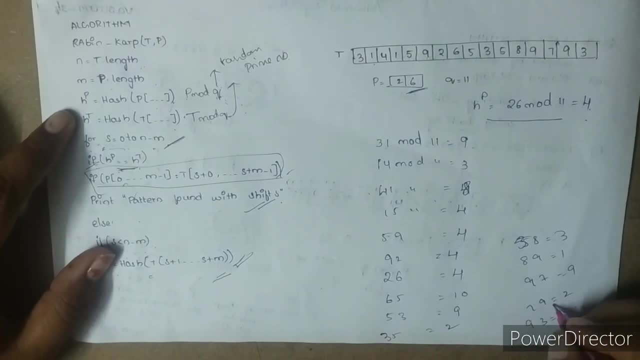 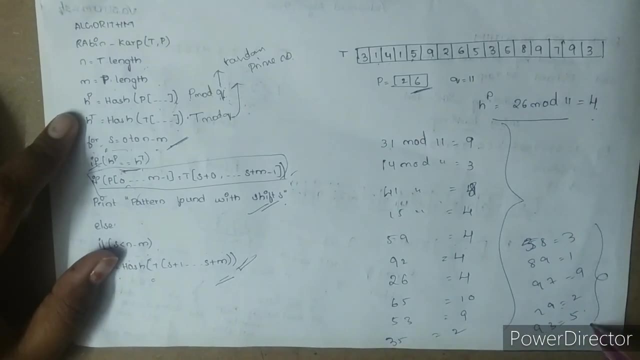 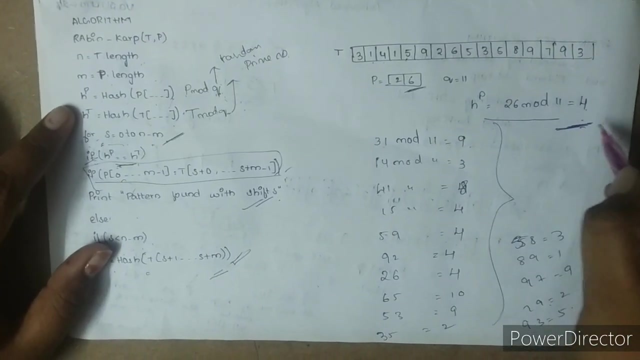 93, equal to 5.. so the shift is here. how many shifts? every single number we have done shifts right. everything single number we have done a hashing and if we have found here the uh hashing number is 4, we have name 4 in these four values right, but we should check whether 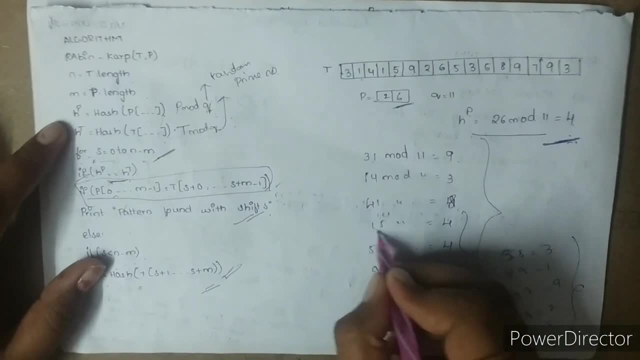 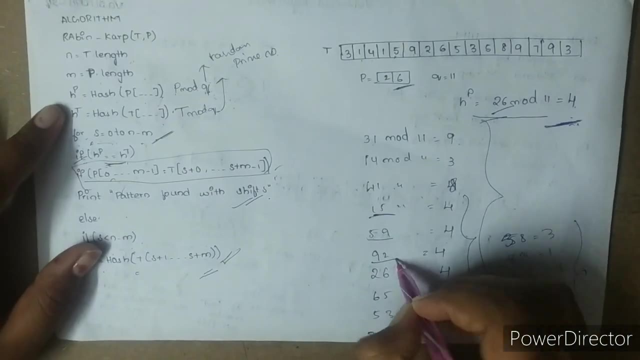 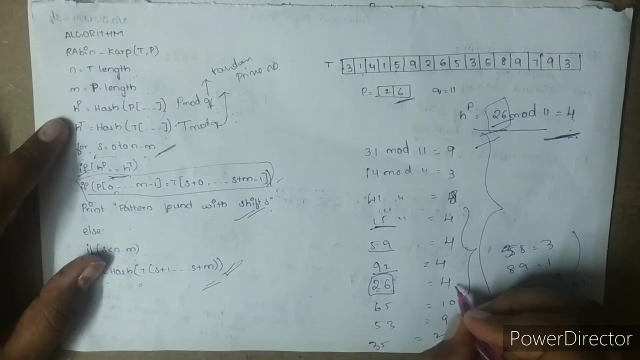 these are spurious heat or valid heat. here, 15 is not matching with 26, and 59 is also not matching with 26, and 92 is also not matching with 26. so but 26, this is the value which is matching with this. so here these three are spurious hits. 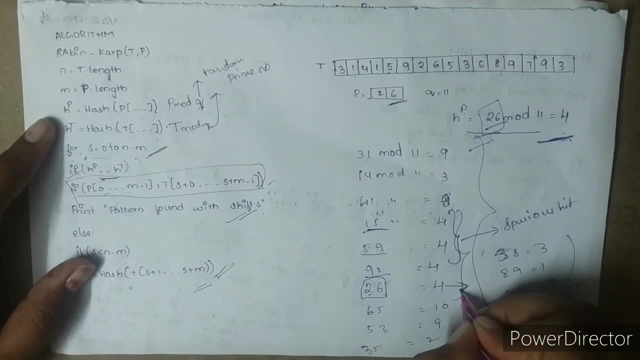 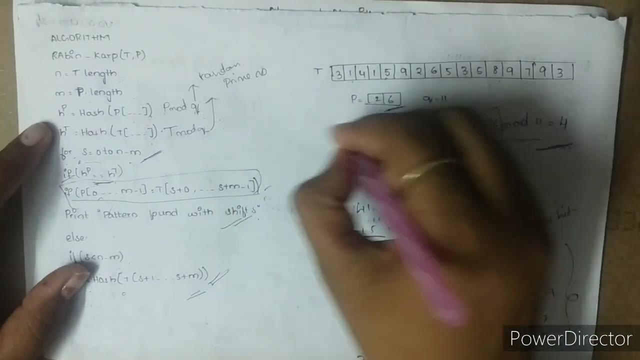 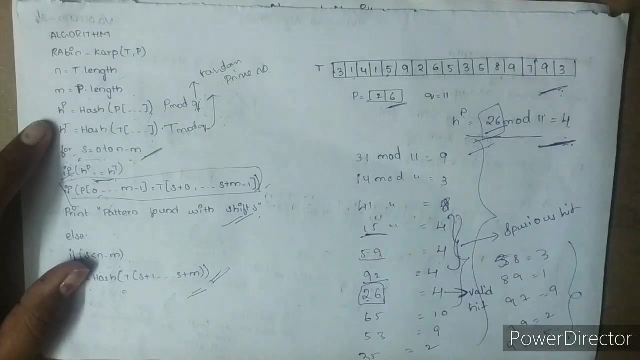 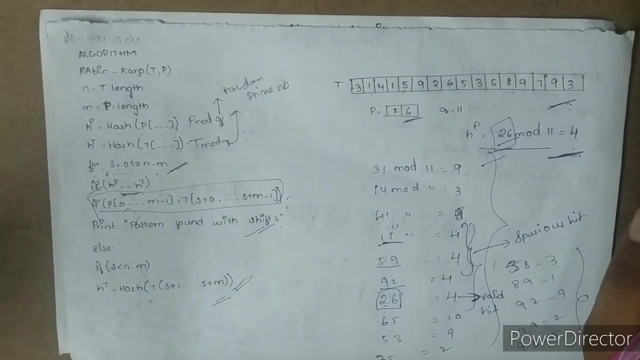 and the last, but one will be valid hit. okay, but we should do, uh hashing. for every single member, for every single number, we should do hashing and then only we should check whether these are getting matched or not. okay, guys? uh, this is a rabin cup method and in next videos i'm going to upload more. 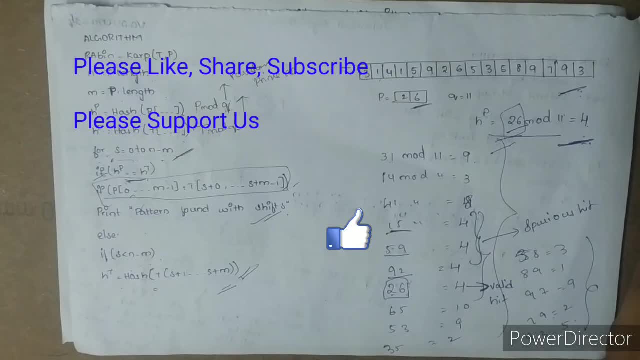 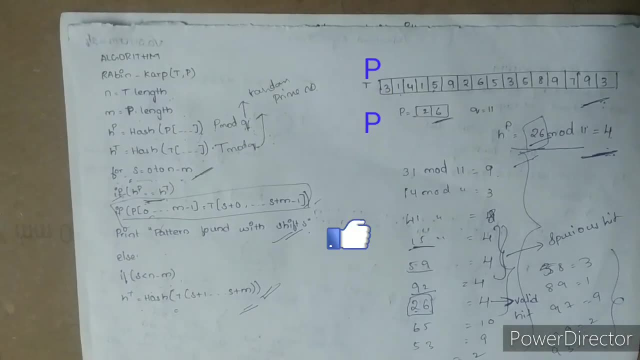 videos on algorithms. so keep watching guys like share, subscribe, uh, subscribe to my channel and i'll see you in the next video to our channel and please support us, thank you.